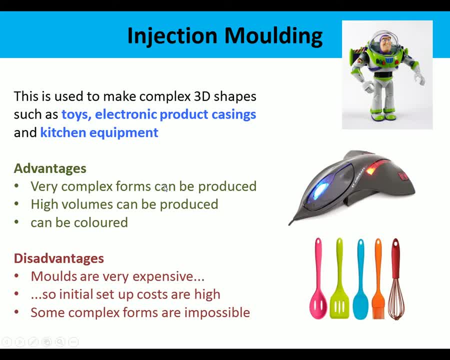 heat. The advantages are very complex forms can be produced, high volumes can be mass produced and they can be self-coloured, so they don't need finishing. Disadvantages are the setup costs and the moulds are very expensive and some very, very complex shapes aren't possible. 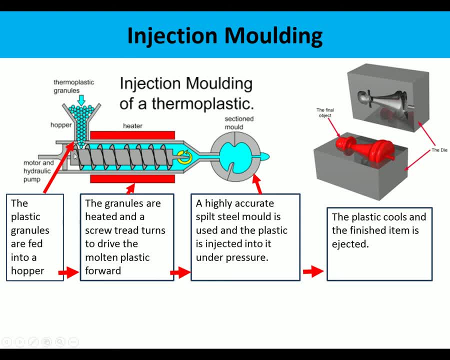 So how does injection moulding work? The plastic granules are fed into a hopper. here It's a picture of the hopper. The granules are heated and a screw- here a screw thread- turns- drive the molten plastic forward. This is then injected into a highly accurate split. 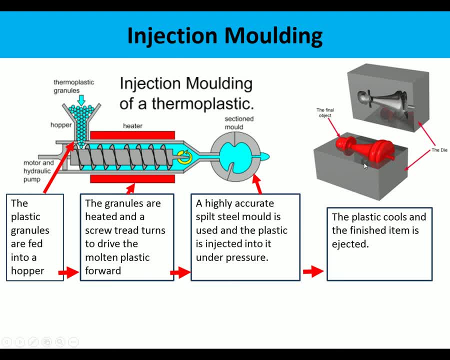 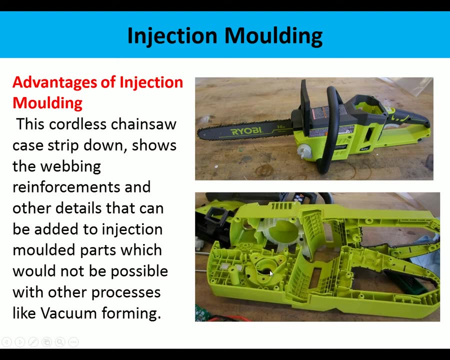 steel mould and the plastic is then allowed to cool, the temperature of the mould is controlled and the finished item is ejected. So these are the stages in injection moulding, The advantages of injection moulding. We can see here a cordless chainsaw and you can see 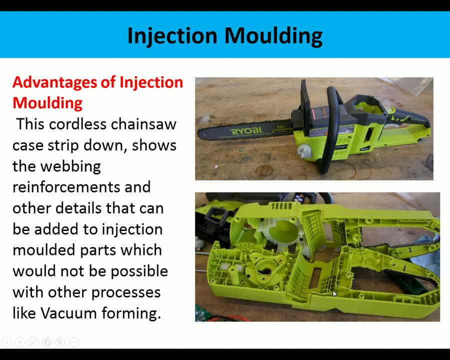 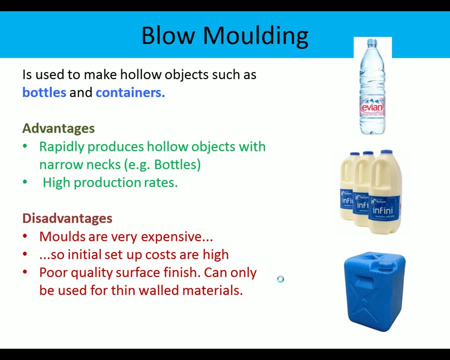 these webbing and these bosses and all this detail, which is only possible with injection moulding. This product couldn't be created with something like vacuum forming Blow moulding. This process is to make hollow objects such as bottles and containers. The advantages are it rapidly produces hollow objects with Narinex ie bottles. so these kind of products. 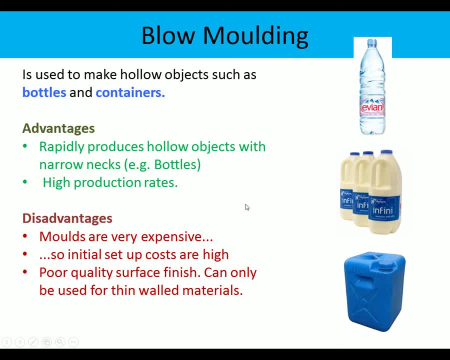 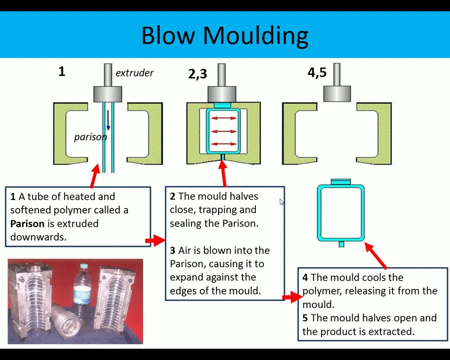 The disadvantages are: moulds are very expensive. again, it's a mass production product. The surface finish is not brilliant and it's only suitable for thin-walled materials, So not as versatile as injection moulding, but a very quick mass production process. Here's a quick description of blow moulding. 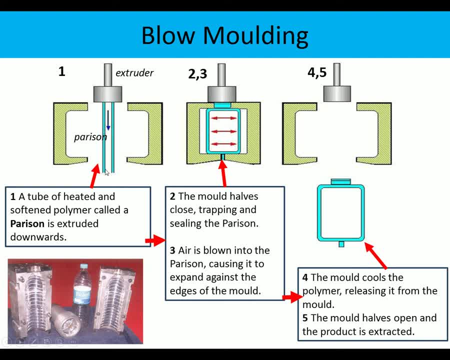 A tube of heated and softened material called a parison is extruded downwards. The mould halves close together, trapping and sealing the parison. Air is blown into the mould and inflates it against the edges of the mould. The mould cools, the polymer is released from the mould, the mould halves open and the product is extracted. 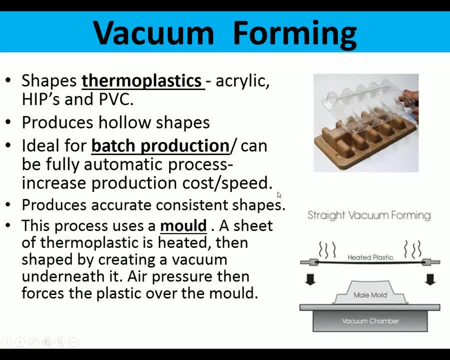 So these are the three stages in blow moulding: Vacuum forming. This shapes thermoplastics, typically acrylic hips and PVC. It produces hollow shapes. It's ideal for batch or mass production. It can be an automated process. It uses a mould and that is placed over. sorry, the plastic is heated over the mould. 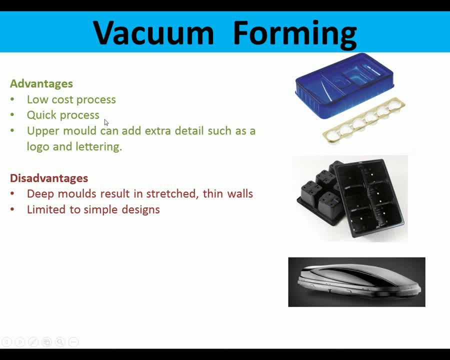 Vacuum forming. The advantages are: it's a low cost process. it's quick. The upper mould can add extra detail such as logos and lettering. Disadvantages: deep moulds. if you have a very deep moulding, it reduces, it stretches the walls. 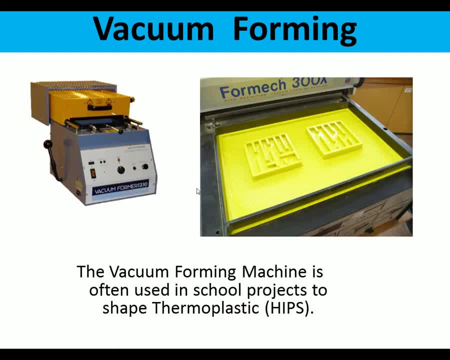 And the shapes are limited to simple designs. Vacuum forming you may have used in schools. It's often used to shape thermoplastic here, such as hips. So that's vacuum forming The process here. we just look at a flow chart of this. 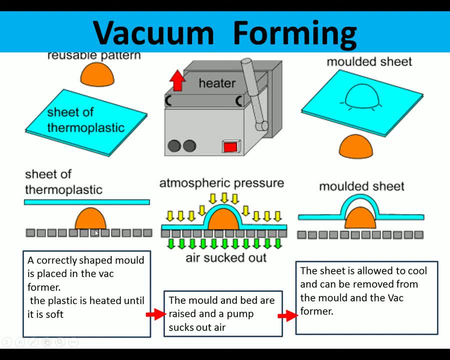 A correctly shaped mould is placed in the vacuum former. The plastic is heated until it's soft. The mould and bed are raised, so the bed comes up, An air pump sucks the air out, Atmospheric pressure forces down on the mould And then the sheet is allowed to cool. 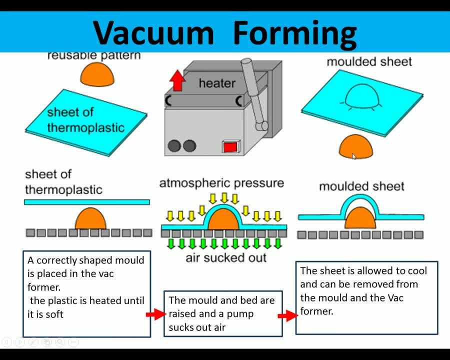 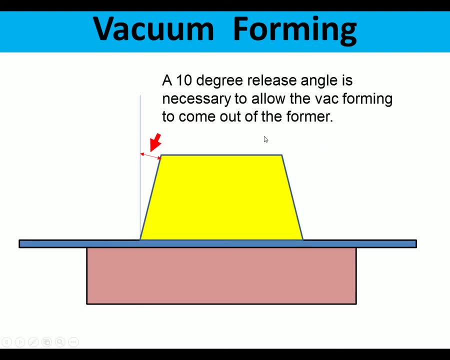 And can be removed from the vacuum former. The mould removed and there's the sheet, often trimmed to size. So that is the process of vacuum forming, Obviously a 10 degree release angle. Here's a close up of the 10 degree release angle that is necessary to allow the vacuum forming to come out of the former. 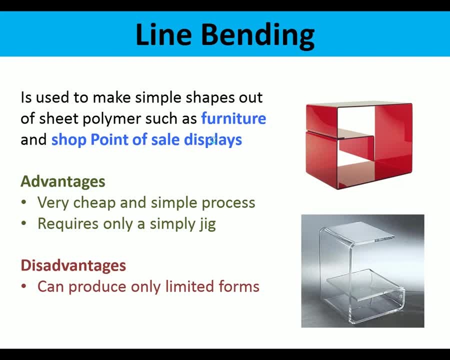 Line bending. This is used to make simple shapes out of sheet polymer such as acrylic. It's used for furniture shop point of sale displays. It's a cheap and very simple process. It only requires a simple jig. But it can only really produce just simple bends. 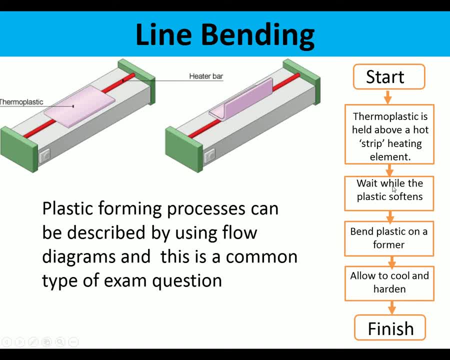 Here's the process of that. We've just got a flow diagram here. Flow diagrams quite often come up for these processes in the exam. So here we've got start. Thermoplastic process is held above a hot strip heating element. Wait while the plastic softens. 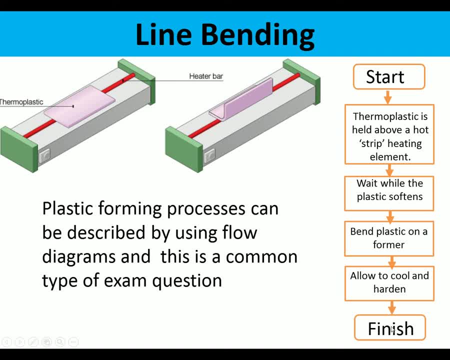 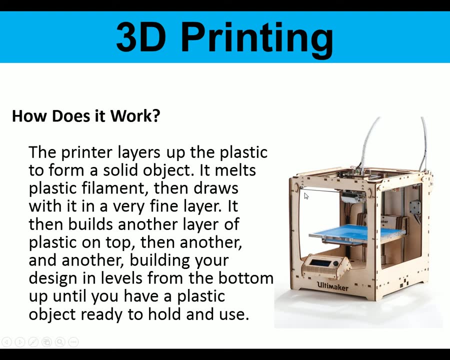 Bend plastic on a former Allow to cool and harden, Finish. This is a basic one that just shows you how you would show this process in a flow diagram. 3D printing. 3D printing is a plastic process. It builds up the layers of a plastic. 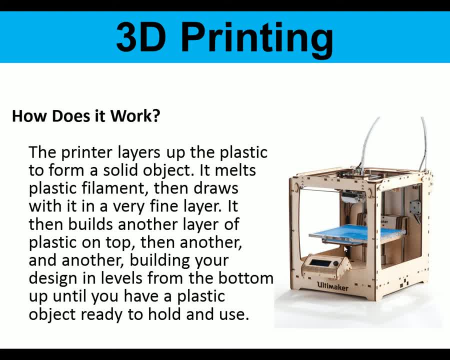 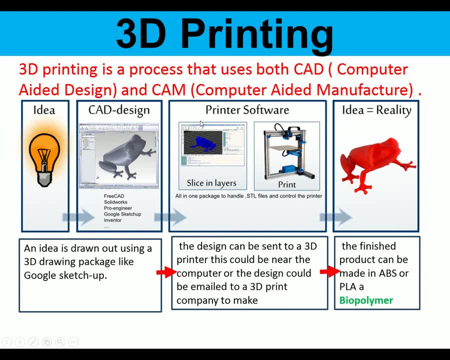 It melts the plastic filament And then just builds up layer by layer, And the bed moves down. So what's the process for this? 3D printing is a process that uses CAD- Computer Aided Design, And CAM- Computer Aided Manufacture. 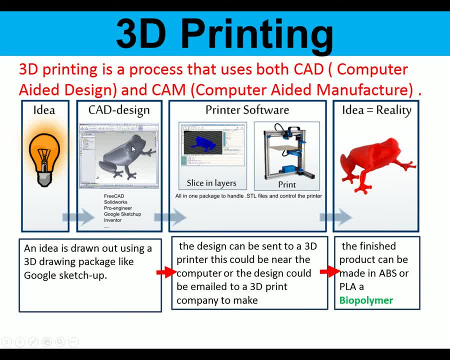 How does this work? Someone has an idea? They draw a CAD design using one of these pieces of software. The printer software actually builds up the tool path or the layers And the design is sent to a 3D printer. This could be near the printer. 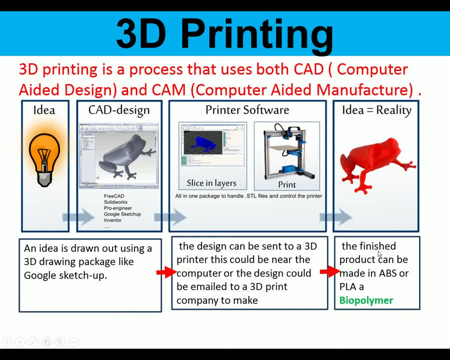 Or could be emailed to a 3D print company to make. Then the finished product can be made in ABS or PLA. We'll look at PLA in a minute, Because that is a biopolymer. So there's the process of 3D printing with CAD and CAM. 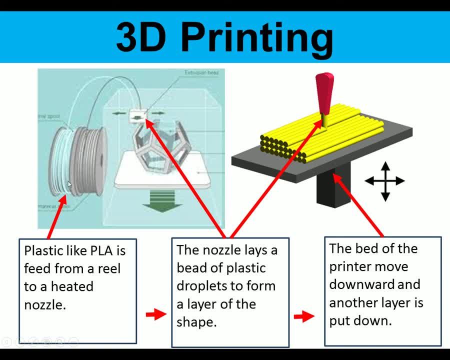 How does 3D printing work? Well, the plastic, like PLA, is on a reel. It is fed into a heated nozzle. The nozzle lays down beads of plastic And these layers are built up. And as each layer is laid down, The bed moves downwards for the next layer. 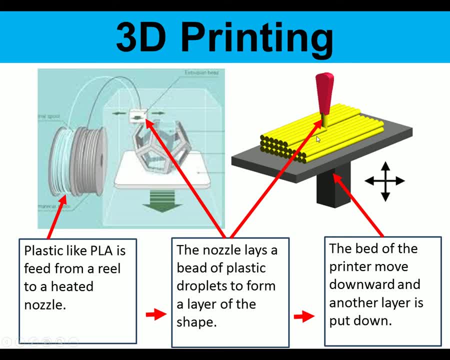 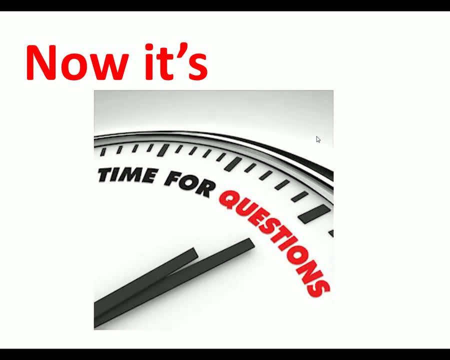 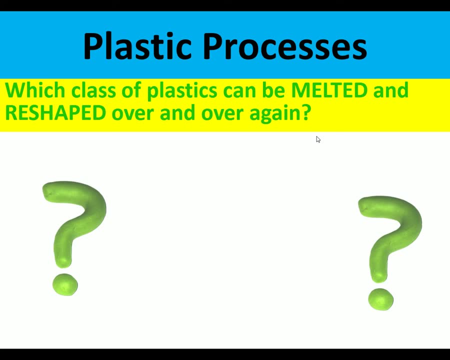 And each layer obviously adheres or sticks to the one above it, And that's how 3D printing works. And that's how 3D printing works. Now it's time for questions. Plastic processes: Which class of plastics can be melted and reshaped over and over again? 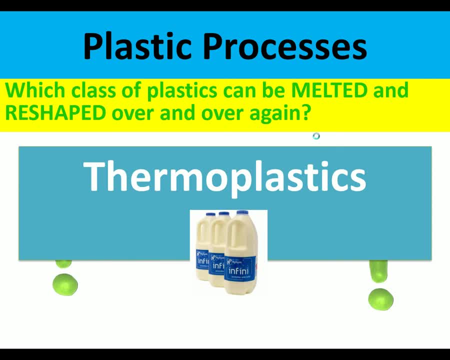 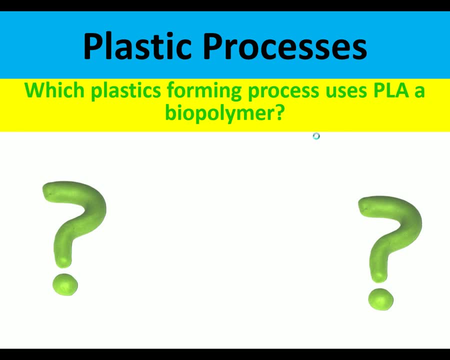 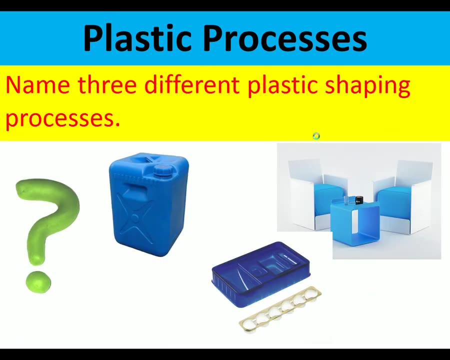 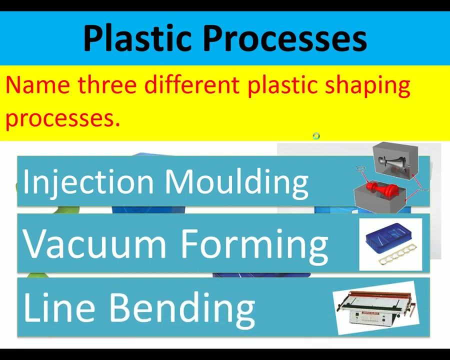 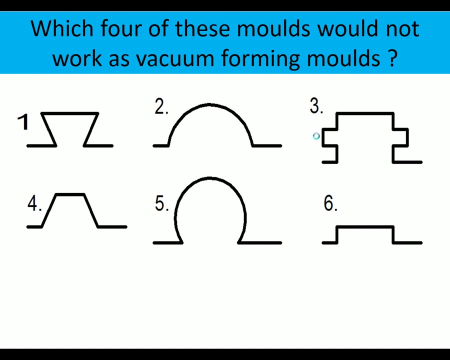 Thermoplastics. Which plastic forming process uses PLA, which is a biopolymer? It is 3D printing. Name three different plastic shaping processes: Injection, moulding, Vacuum forming And line bending. Which four of these moulds would not work as vacuum forming moulds? 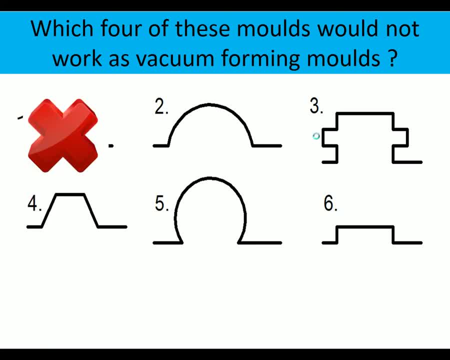 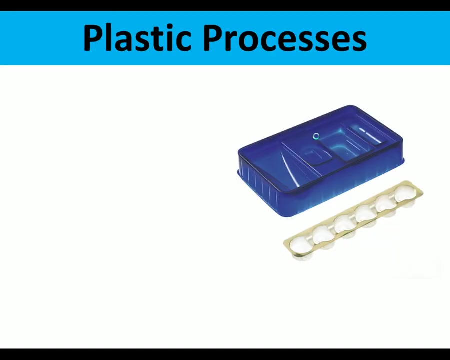 Number one: No. Number two: Yes. Number three: No. Number four: Yes. Number five: No. And number six: No. Remember: vacuum forming. moulds need a release angle to work properly. Plastic processes: This was made by vacuum forming.